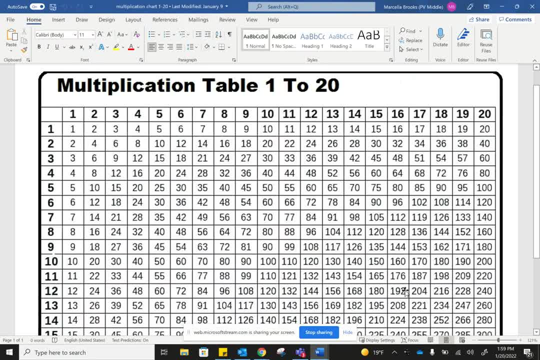 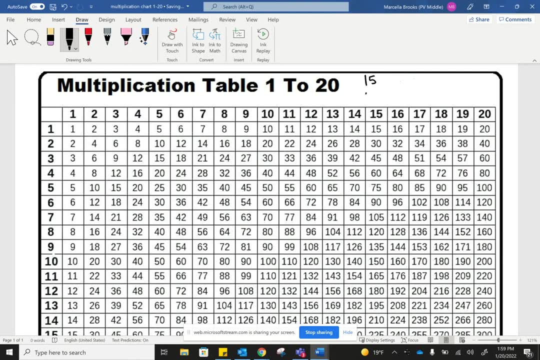 This is a video on how to find the GCF, or greatest common factor, using the multiplication table. So let's say I want to find the greatest common factor of 15 and 10.. So I'm going to go first, I'm going to start with 15, and I'm going to circle all the places that I see 15 inside of the table. 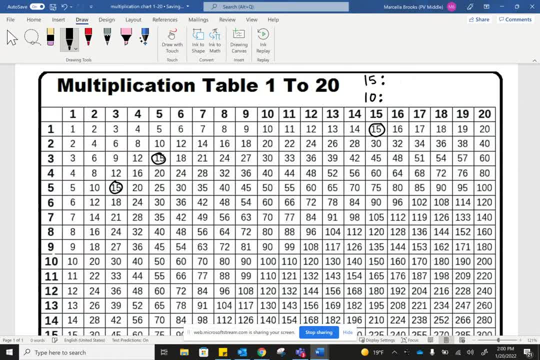 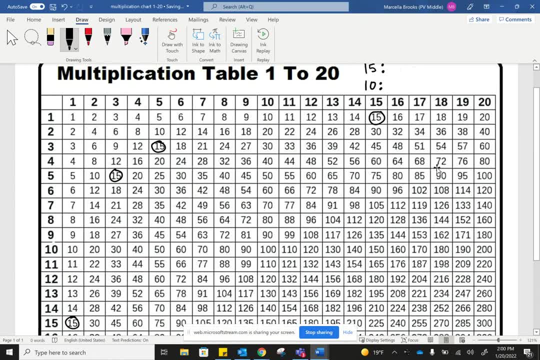 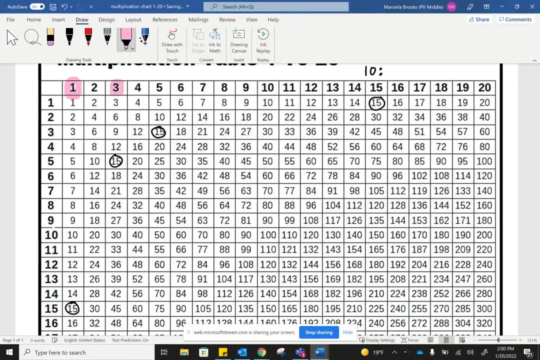 Okay, Okay. so that means that I have 1 circled in the 1 column. that means 1 is a factor, 3 is a factor, 5 is a factor and 15 is a factor. Those are all the factors of 15.. So 1, 3, 5, 15.. 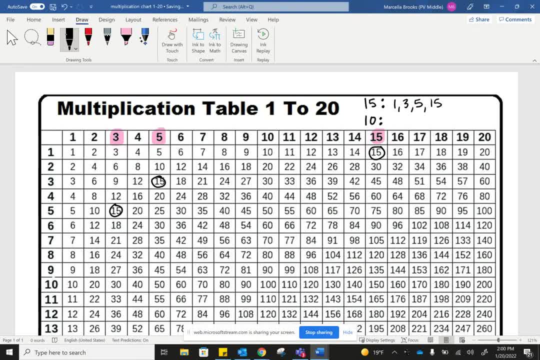 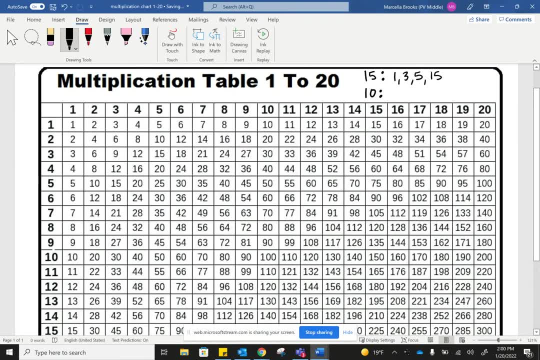 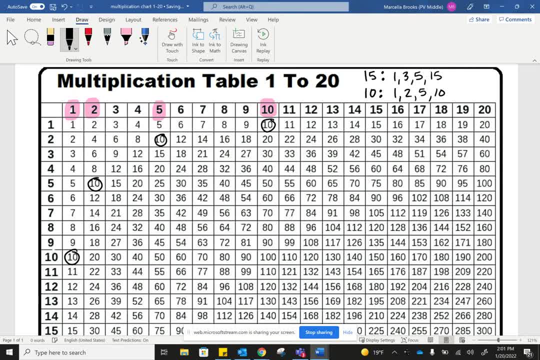 So they both share a 1,, of course, and a 5.. So my GCF is 5..